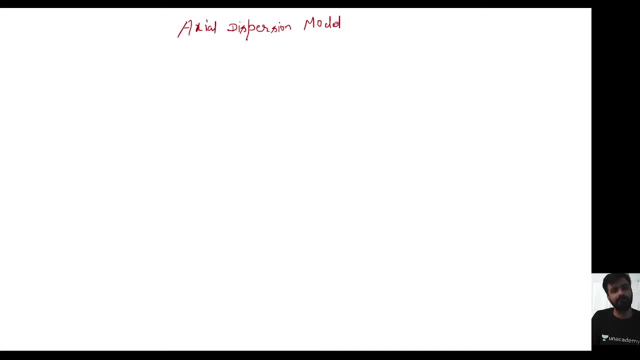 So, my dear students, you can see, the importance of this model becomes very important when we talk about the plug flow reactor also. So this model is also valid for plug flow reactor. First of all, plug flow reactor. When we talk about, my dear students, ideal PFR. 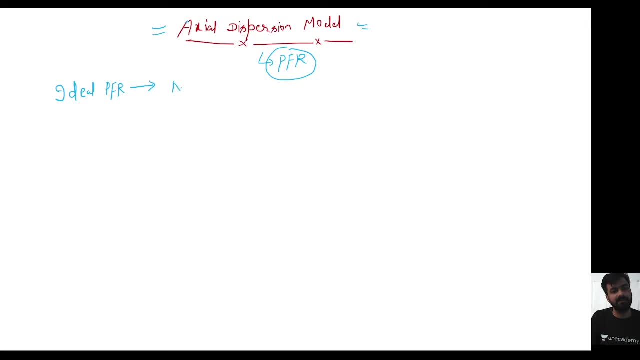 Ideal PFR. there we assume that there is no axial mixing possible in ideal PFR. No ideal mixing is possible in case of ideal PFR. That becomes very important. But whenever we talk about- you know, my dear students- reality, in the real case, there is no such thing occur. 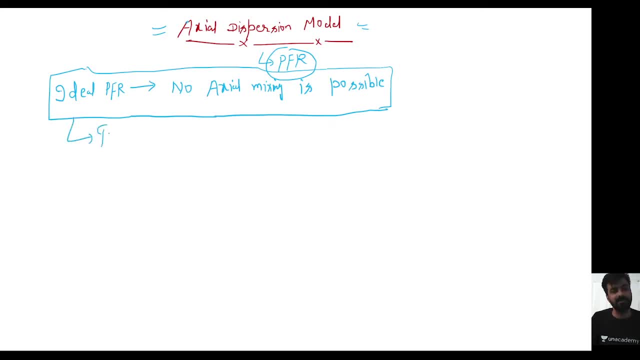 you know, in PFR, In PFR also. So when we talk about the real case, when we talk about the real case, there will be some non-ideality that will get arrived, OK. so the real case is non-ideal reactor. 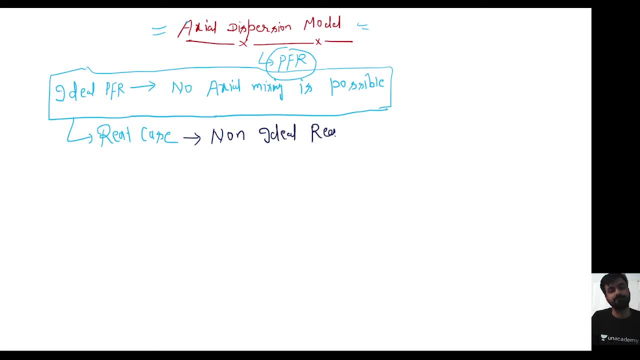 OK, so whenever we talk about the real case, that is, non-ideal reactor, like you know, when we talk about non-ideal gas, so non-ideal gas also, you know it's perishable after that, you know exist in their nature. 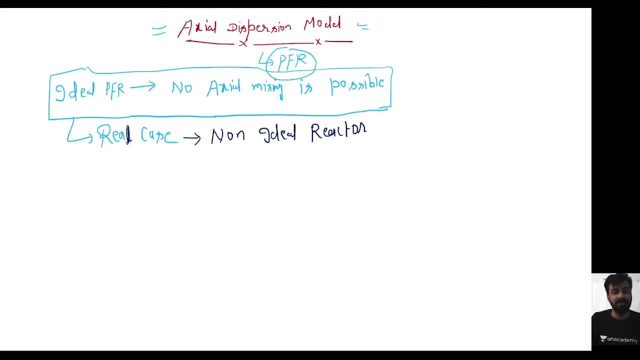 That is actually so sweet. OK, so A particular condition of real gas becomes ideal gas. OK, so here also at a particular condition ideal. ideal I mean in a real reactor. we become ideally, And the assumption is: no, I'd maybe, if possible, then that will meet the really Oh yeah. 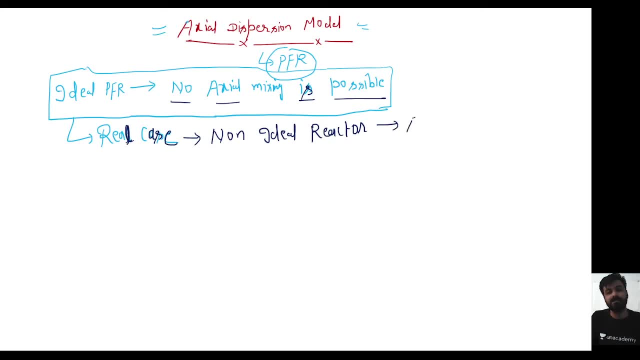 Oh yeah, So So yeah Again, The Indian case, The Yeah, Oh Yeah, So, Oh yeah. Then will be an axial dispersion will be possible. Axial dispersion or axial mixing- is there? Axial dispersion and axial mixing- is there, my dear friends? 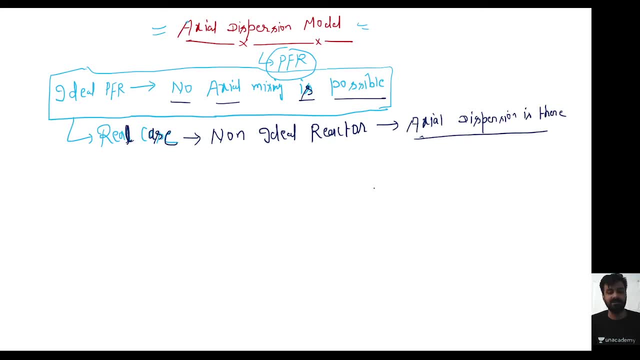 So the I mean whenever there is an axial mixing, that axial mixing, you know term, encountered by a term that is called an axial dispersion coefficient. okay, So definitely, you will have to add some terms over there and that term is called as the axial dispersion coefficient. 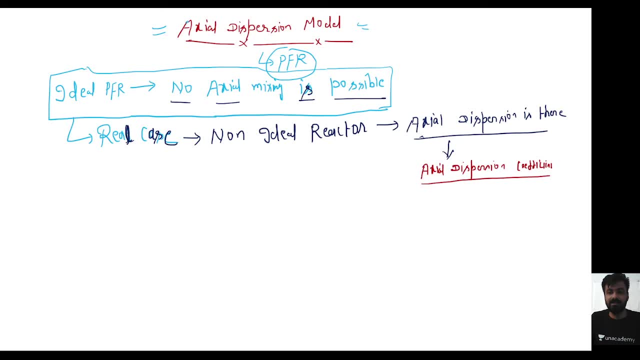 Now you are getting what I want to discuss over here. There is term that you will see in the derivation: there will be an axial dispersion coefficient, okay, So you know it is same as like diffusion coefficient, and also it is follow fixed law of diffusion. So same as. 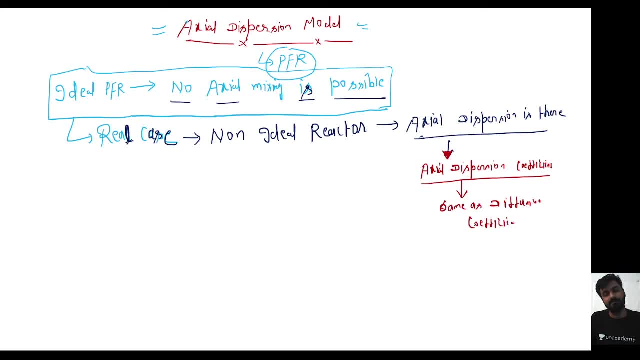 diffusion coefficient and it will also follow fixed law of diffusion. Are you getting fixed law of? it will also follow fixed law of diffusion. So I think up to this. it is very clear whenever we talk about the real reactor. this is the case of non-ideal reactor, and in non-ideal reactor axial dispersion will be. 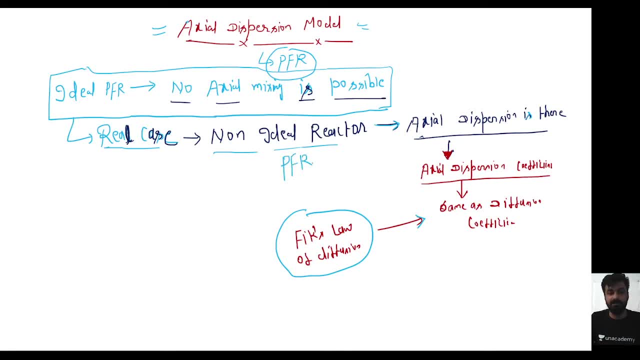 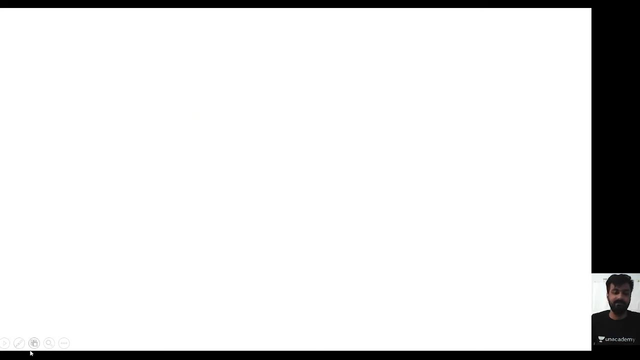 there in case of PFR also. I am only talking about PFR, okay, not talking about MFR, because this model is valid for PFR. okay, PFR, So axial dispersion coefficient will be there. okay, and that axial dispersion coefficient behaves like a. like the same. the axial dispersion coefficient is same like. 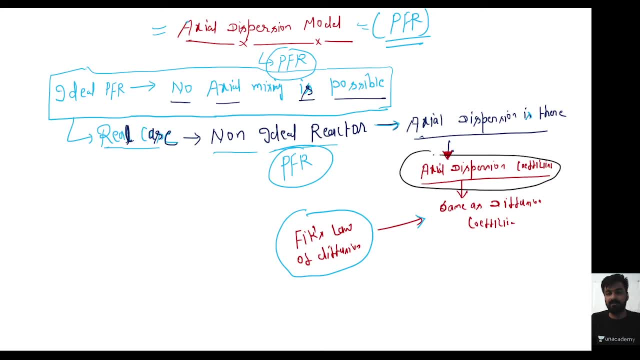 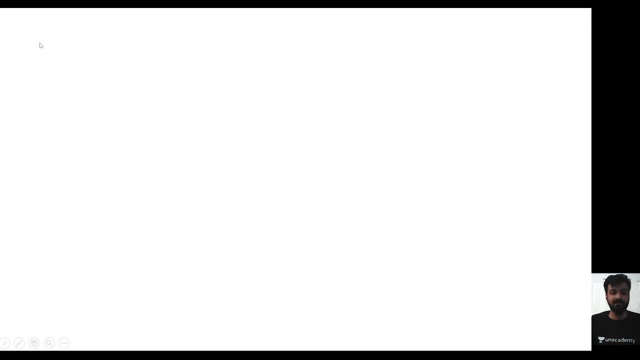 if you know your diffusion coefficient and it will also follow my description: fixed law of diffusion. So it will also follow my direction: fixed off diffusion. I think up to this. every one is clear now. Now, coming to the next one, how it is behaving like So: meditation when 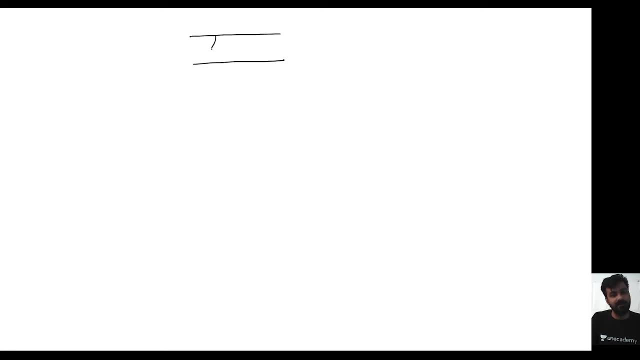 we talk about pooled flow reactor, the case of plug flow reactor in profile of priority, but when we Сm of plug flow reactor is like this: it is come thoroughly flat profile. okay, this is thoroughly flat profile, it is ideal PFR, but in reality, what will happen? 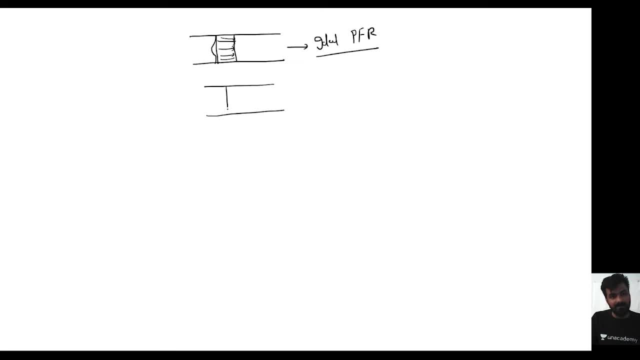 there will be some dispersion will be there. are you getting? so here you can say the profile should be like this, but in real case it does not look like this. so there will be an axial dispersion like this and it is called axial dispersion. are you getting? this is axial dispersion. okay, now how this axial term? 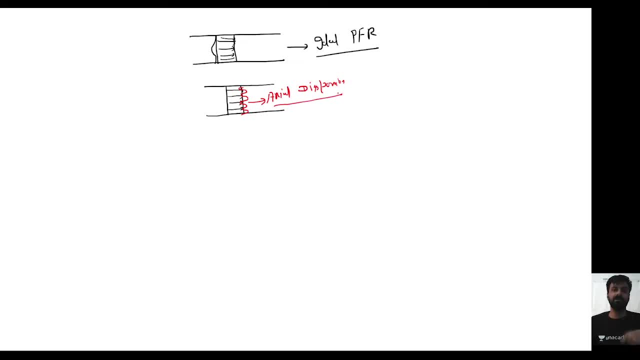 axial dispersion term will be, you know, encountered in the mathematics. that is the objective of this session and I will let you know later how we are going to encounter this axial dispersion term and how I mean, our PFR get deviated from, you know, ideality due to this axial dispersion. so 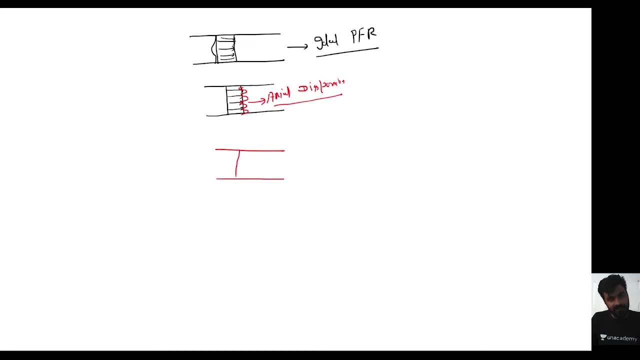 just try to understand one thing. I am starting this, the mathematical modeling of this part actually. so I am assuming this is flat flow profile. okay, so here molar flow rate of tracer will be entering FA at z, and here I am assuming a small flow. so we as a 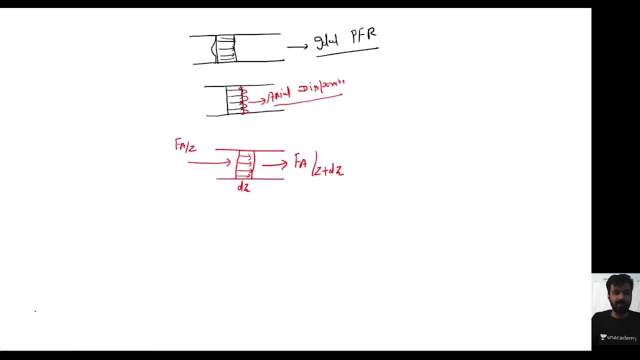 uh se estabilizar bulk flow and way there are altered. briefly, level here thats another flow plus a bulk flow flow here is defined below raining a down, not even falling down. a gonna be very similar and the last in the long term flow is modified. also, and this is books per unit, it is the anderen one and the last that is display in this writing. that is Friday. after that it will sustain b s card here. so you find both: scallαι, arriveaded to Paris, okay, and yeah it will be leaving, okay, and here it will be living at a fear, at okay, a z pluselle, okay, and it is bulk flow distribute and here it will show bulk flow because there is. 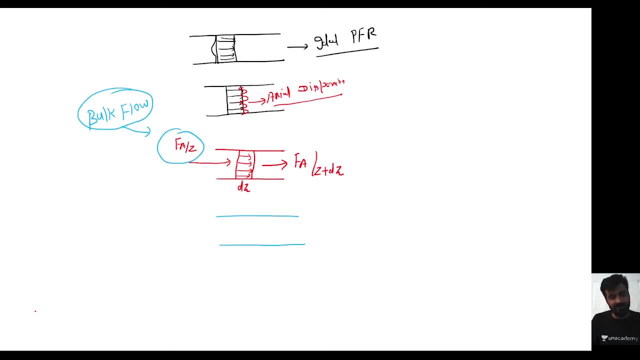 ship flow, that already i have told you that- because due to dispersion, so that terms will become also important in case of non ideal reactor and which is absence in case of ideal reactor. so here, so it will be like this: here it is dispersion, so this term will also come in importance. so here, 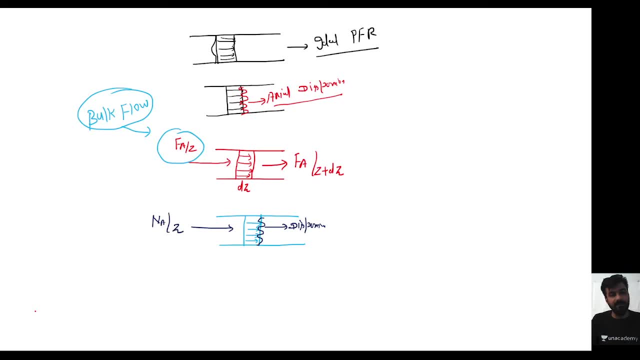 it will be going at na at z and here it will be coming na at z plus d. that, if i am assuming. the thickness, are you waiting? and here it is dispersive flow, are you waiting? because both of these two will have to come, you know, considered in the model whenever you are. 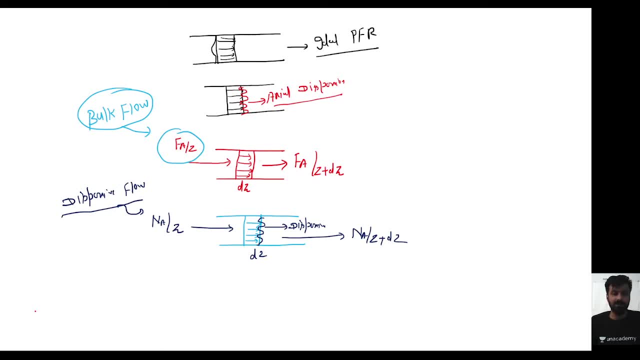 going to model the pfr and that actually known as vr. so here the unit of this particular thing is mole per second, because it is molar flow rate. and here, when we talk about migration, bulk flow, one thing i am letting you to know: bulk flow model, here, f, it can be determined by, you know, volumetric flow rate into cross. 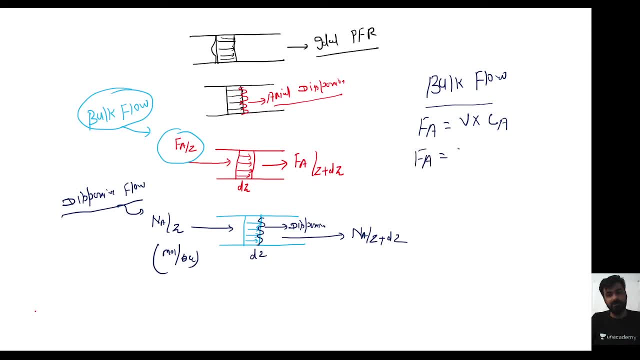 sectional, sorry, concentration. so can i write f page costumization? you multiply with area, that is volumetric flow rate and it will be multiplied with ca. are you waiting? say simple, like that. you all have started in. you know mass transfer course, so it will be very easy. 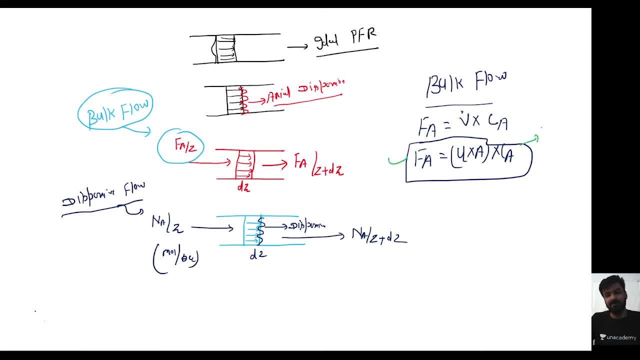 for you to understand the thing. so it is bulk flow. this term signifies bulk flow, and already i have told you that this term- dispersive flow- will follow fixed law of diffusion. so can i write na, that is equals to my distance, and then multiply with a, that is: 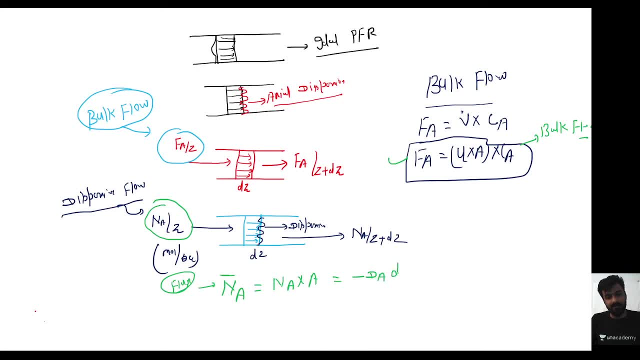 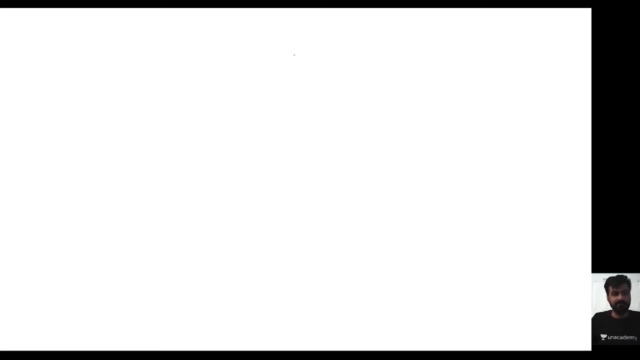 so that is equals to my descent, minus da dca by dj, and multiply with area. are you waiting? you can understand these things from here, so we have calculated both of them now. coming to the next, now apply for the tracer balance. okay, you can understand the thing. 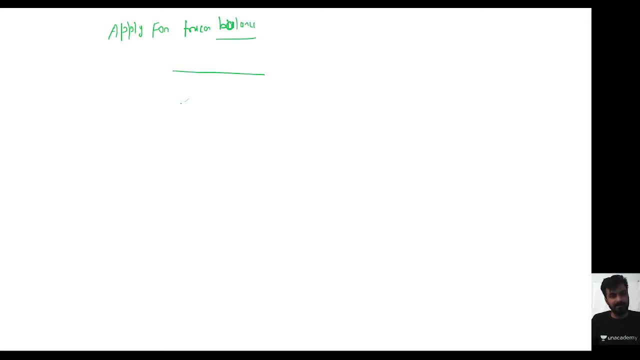 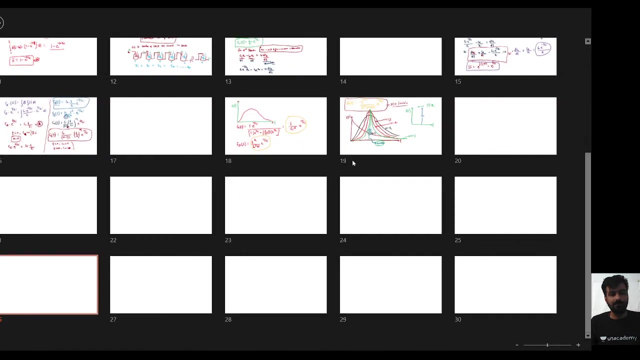 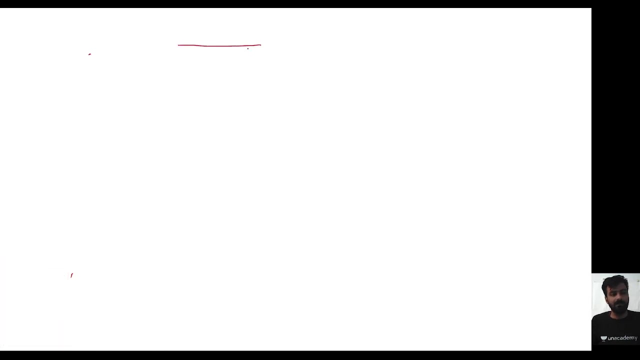 operation. when we apply the tracer balance here you can understand the thing from this particular cross sectional era. what will happen? concentration multiply with a multiply, you at z here and here. this is bulk flow. there will be two flow over here. one is bulk flow and one is dispersive flow. okay, so here. 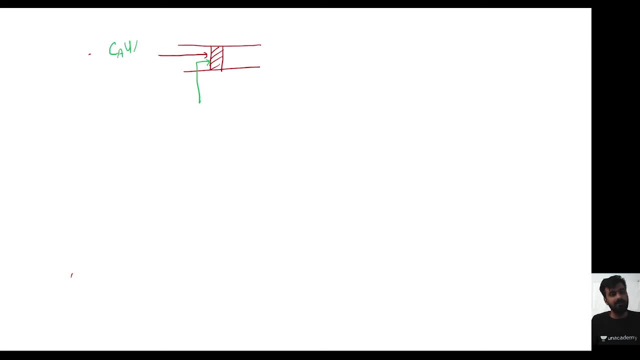 it is ca? u and cross sectional area, and here my direction na bar at z and here it is at z and here it will be coming ca? u at z plus dz and here one more, na bar at z plus dz. are you getting both of these two things will get coupled when i will. 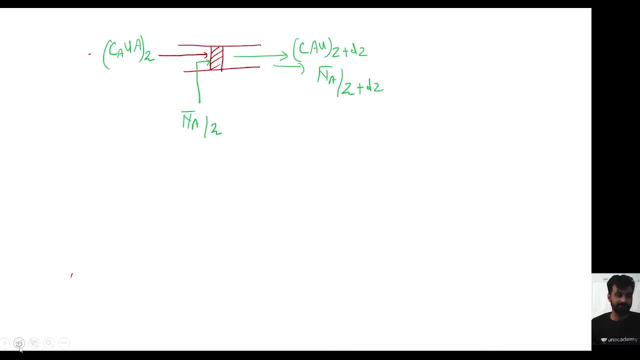 be doing the modeling of this pfr now coming here. what happens over here? so can i write my notion: fa at z plus na bar at z. are you getting? that is tracer in minus minus. fa at z plus dz. are you getting minus na bar at z plus dz? are you getting minus na bar at z plus dz? are you getting minus? 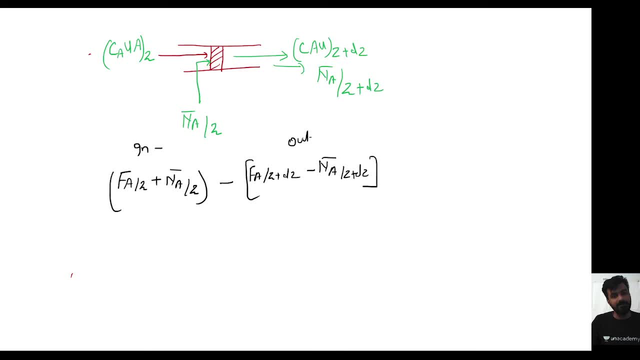 z plus dz that is out in minus out, okay, and that is equals to accumulation. so d upon dt of ca, ca, okay, and dz in minus out that is equals to. this is simple mole balance over here that i have used. okay, so can i write fa at z plus na bar at z, okay, and i'm 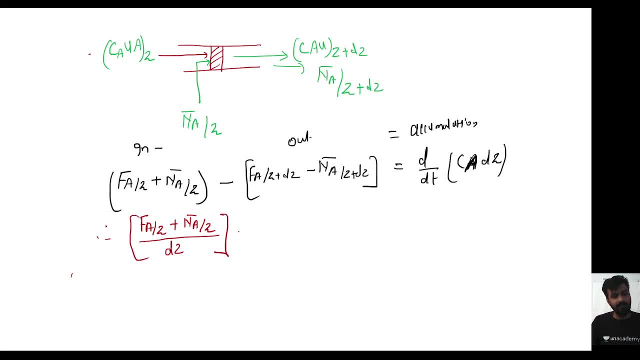 just dividing this term by dz are you getting minus fa at z plus dz, minus na bar at z plus dz. divided by dz, that is equals to a and dc by dt, and here dz term i have divided, so it will come like this: okay, so again can i write here: minus dfa by dz, minus dna bar upon dz. this is just the simple. 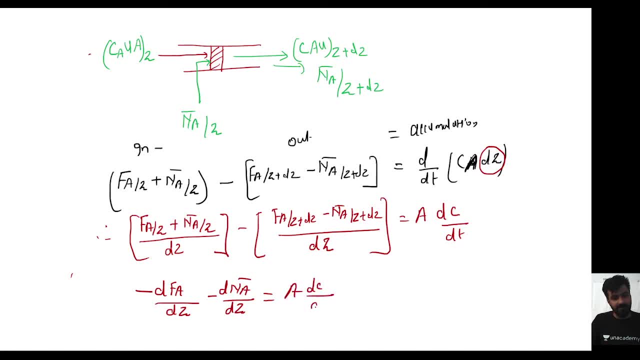 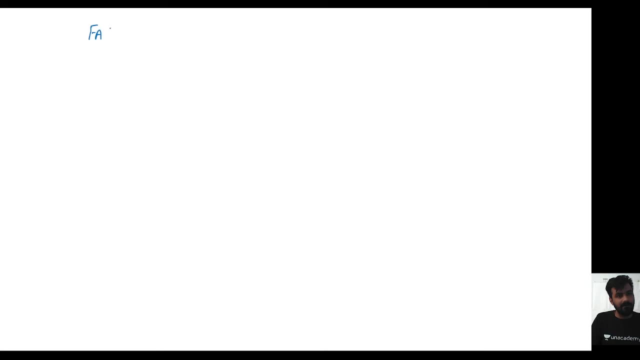 differential that is equal to a dc by dt. so again, here can i write f a, and that is equals to c and u a. this is bulk flow. so ca i write here: minus쿉 a, muss you dz, arhn k, arhn k, Vivian, it is so. it gives me mu of 2 отпurussia bar, so this is bulk flow. so can I write here minus A u dz, because this is bulk flow. so can I write here: minus A u dz, because this is bulk flow. so can i write minus a u dz, then inducing mu guilt. so again is the only value here. so this is only function that we are doing and we are going to write again in these conditions. this solution, fuckper puzzle, is also of Enter for. 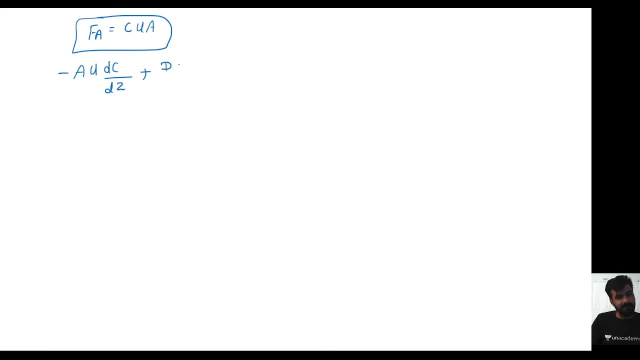 DC by DZ plus D del 2 CA upon del Z2. that is fixed law of diffusion that will follow. multiply with area that is equal to A DC by DT. are you getting so can I say, this A, this A and this A will get cancel out. finally, you will be getting a. 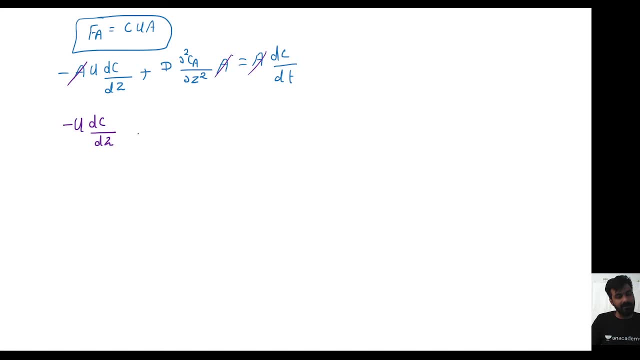 derivation U DC by DZ plus D del 2 CA upon del Z2, that is equals to my derivation del CA upon del T. it's a very important relation and this relation is called equation for dispersion model, equation for axial dispersion model. now, what you can, you know, elaborate from this particular 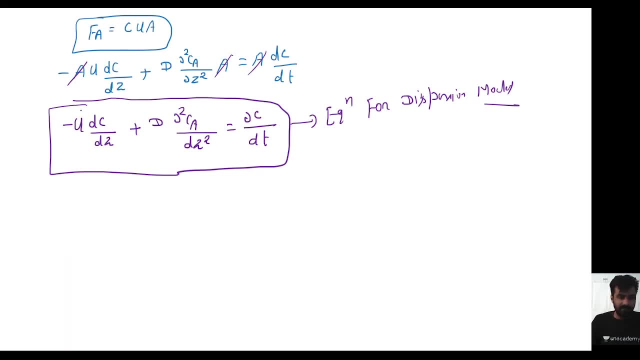 equation. so here you can see this is term of bulk flow. this term signifies the diffusive flow in a unsteady state condition. are you getting so when we will change in dimensionless parameter? why we change dimensionless parameter in dimensionless parameter? because the thing will becomes very easy for you to 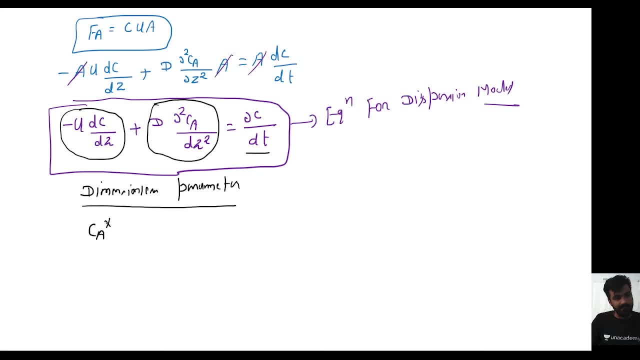 understand or remember. so can I write here CA star. that is equals to CA upon CA. naught, okay, CA star is equal to CA upon CA. here you can write this concentration as CA also, because it will become very easy for you to understand. okay, CA del CA. here you can write CA. it is CA if a reaction is happening from A to B. 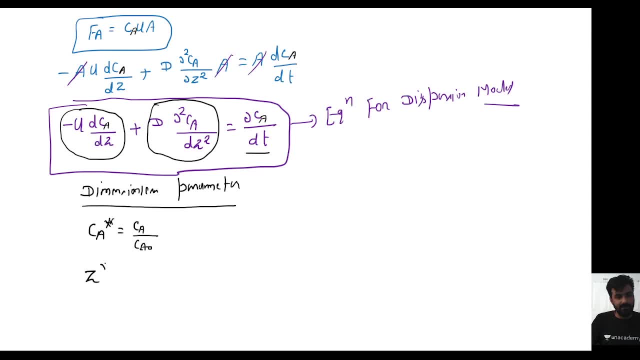 okay, that's fine. and Z star that is equal to Z upon L, where L is length of P of R, throughout the length it will cover. so if it will be our P of R, so this length should be there to cover this particular reaction to product. okay. 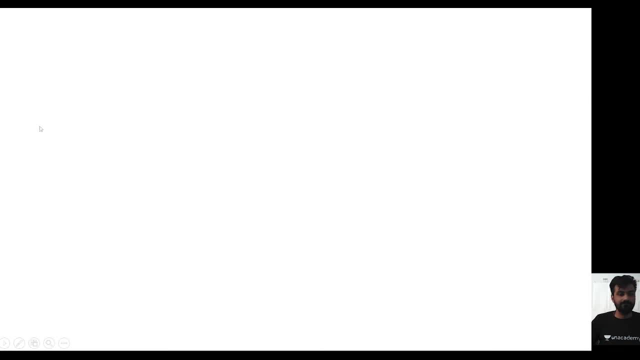 throughout the room. so and can I write time that is going to tell upon you length of PFR, upon velocity of the substance coming. so can I write my destination minus u CA naught upon L and del CA star upon del z star, plus d CA naught upon L del 2 CA star upon del z star that is equal to u CA. 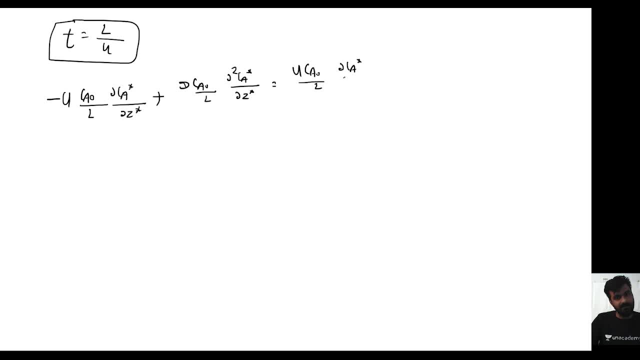 naught upon L and del CA star upon del t. only I have put all these things over here. I am NOT doing any new things. that now, finally, you can write this term: minus CA: naught del CA star upon del z, star plus de upon ul. then you can write del 2 CA. 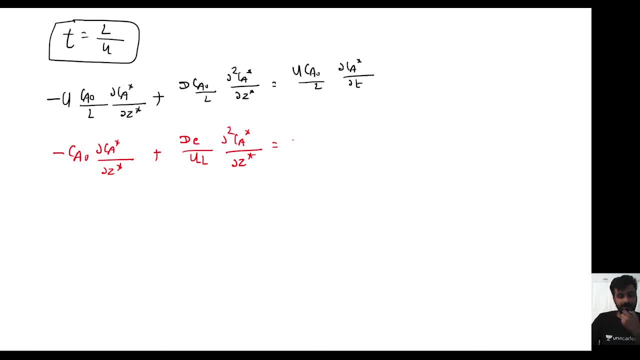 star upon del, z star that is equal to del, c star upon del of the value and minus the difference between Z 가자 1 350. Behind you before I shall be shallowly So. when you say footage this, and I think the e upon u, you cannot predict in terms of the direction of the body. 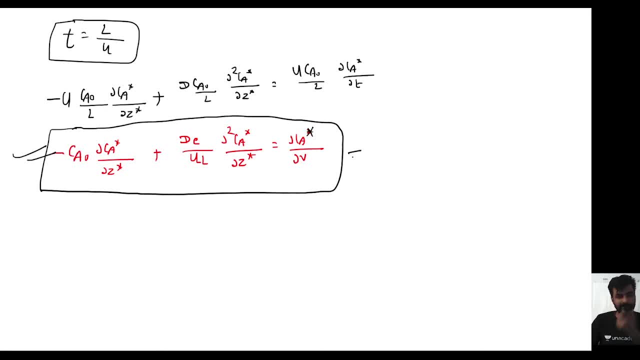 in terms of distance. if it is parallel, it is the third particle in the v you will be writing. now let us take this dashed diagram you can see over here. let's write that we are going to see much bigger in the dimensional live classroom. so if everybody boiling is automatically 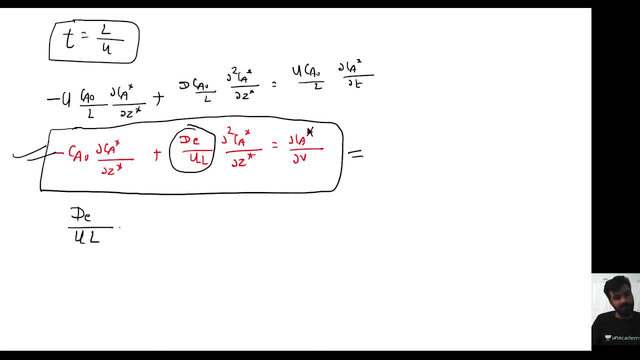 the term DE upon UL. okay, that is called as dispersion number, very important number. that's why we have put in the form of dimensionless parameter, and that is equals to transport of tracer due to dispersive flow, divided by transport of tracer due to bulk flow. 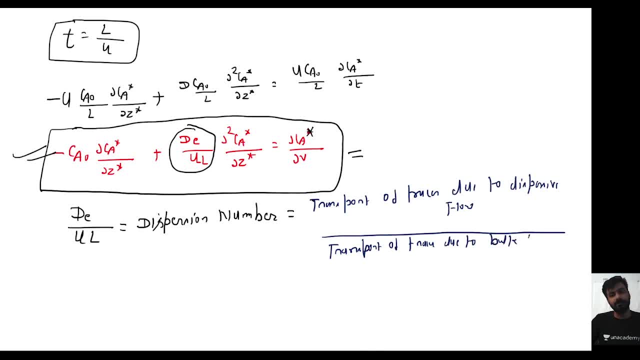 are you getting now what you can deduce from here, my dear friends? if dispersion number exist, if dispersion number exist, then what will happen? the reactor will be non-ideal. are you getting? because here the dispersive flow is also coming in account, so that 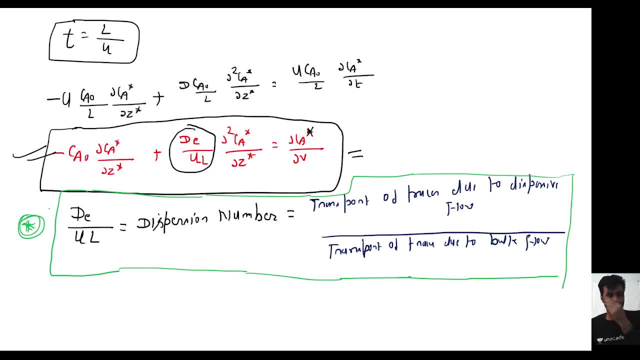 the reactor will become non-ideal. so if you want to check whether the reactor is ideal or non-ideal reactor, you just go for calculation of dispersion number. if it is going to exist- and this shows the significance of dispersion number- is the transport of tracer due to dispersive? 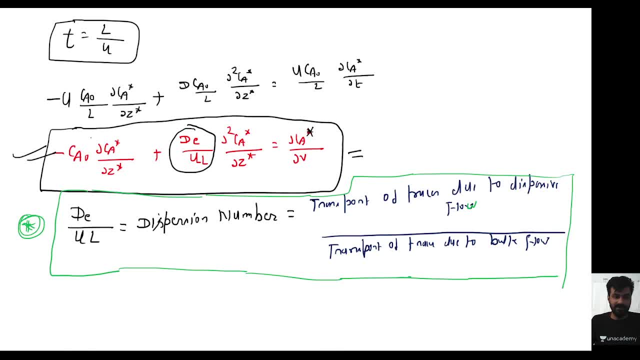 flow and upon transport of tracer, of tracer due to bulk flow. you can say here: D signifies the dispersion and U in multiplied with L signifies the axial flow. that is bulk flow. okay, bulk flow, sorry. now so I can define dispersion number. 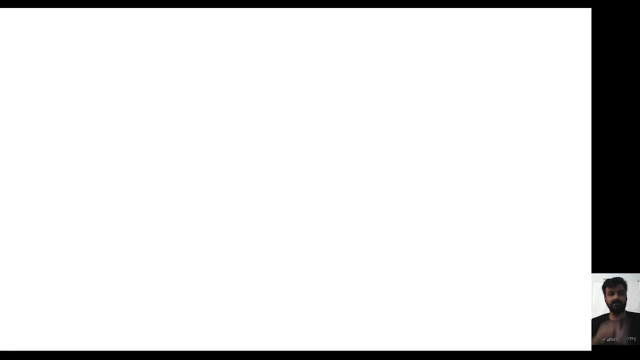 is a measure of relative importance of transport of tracer due to, you know, the dispersive flow and over the bulk flow. okay, so you can define the dispersion number here. also, it shows the relative importance of tracer, relative importance of transfer of tracer. it will become important. 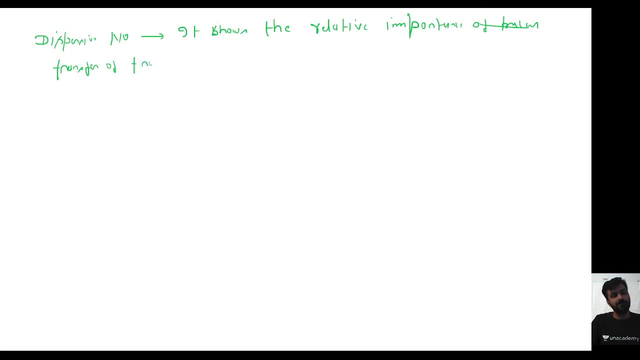 transfer of tracer due to dispersive flow over bulk flow. okay, I think the definition part is very clear to all of you and my dear friend. it's very important definition and it's very important parameter in most of the interview. interviewer try to you know, trap you. 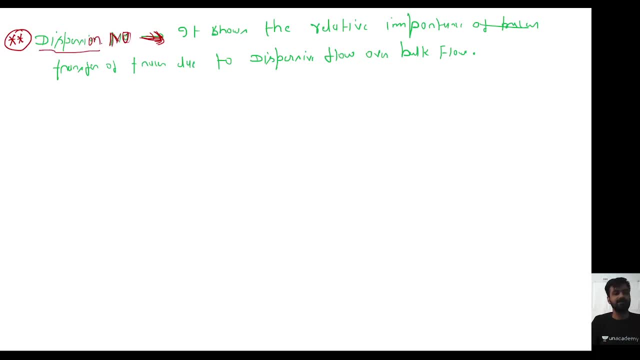 while asking all these things. okay, so dispersion number. most of the student use to left this particular part, but this part is not very tough already. I am, you know, trying my best to let you understand this part exactly. okay for the non ideal lecture. now coming to the 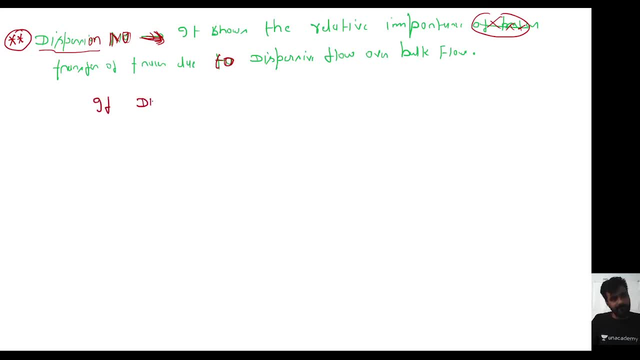 next part. it's very important. if this person number is equals to zero, what does it mean? that means transport of tracer due to dispersive flow will be equals to zero. are you getting? transport of tracer due to dispersive flow is equals to zero. 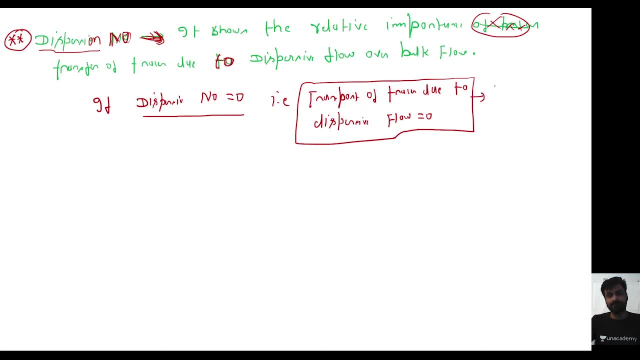 okay, and or you can like, flow is only due to bulk flow term. are you getting? these two things can come into account whenever dispersive flow is zero. sorry, dispersion number is zero, so this will signify. in the case of when dispersion number is zero, it will signify. 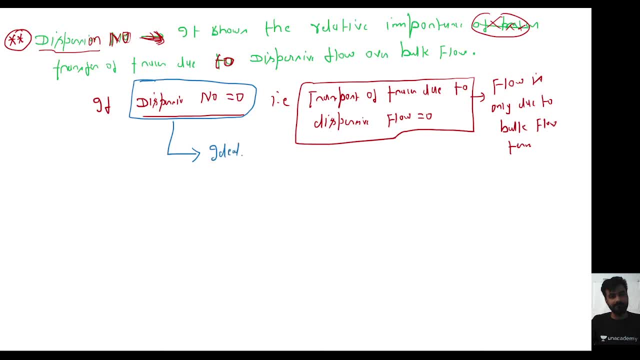 the ideal, ideal, ideal, ideal, ideal, dispersion number will be there. so don't get confused here. if they will be asking if dispersion number is zero, then you will have to understand that you have to say that ideal. this will be the case of ideal plug, flow react and when. 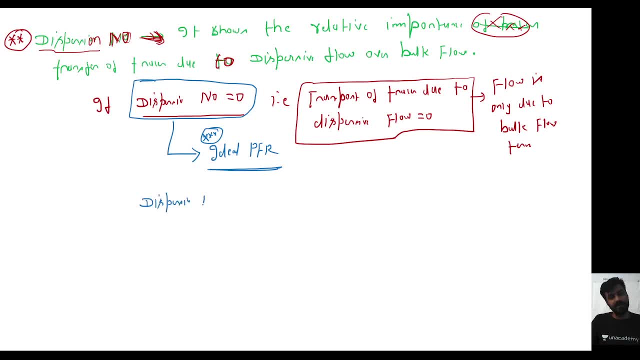 you understand dispersion number that is equals to infinity. so what will happen? transport of tracer is due to only dispersive flow. transport of tracer is only due to dispersive flow, and what does it signify? it signify it is the case of ideal CHTR. okay, it is very important point. 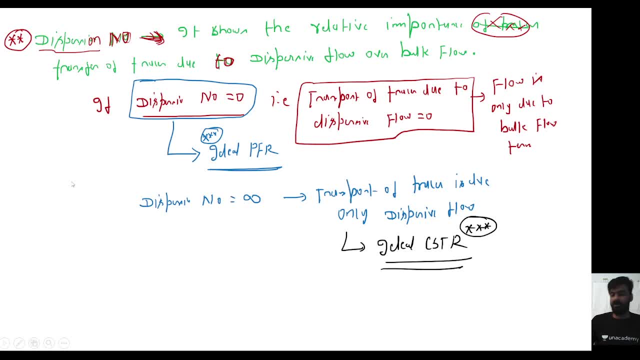 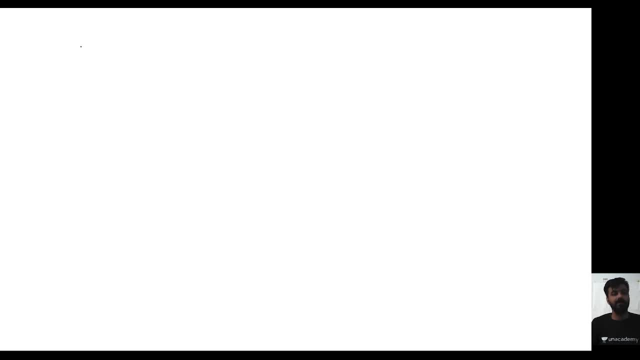 that you have to keep in your mind whenever you are going to give your interview in any public sector and in any company. okay, so now, one more important factor that has been left in this session is that is patulate number. patulate number and that is equals to 1 upon dispersion number.